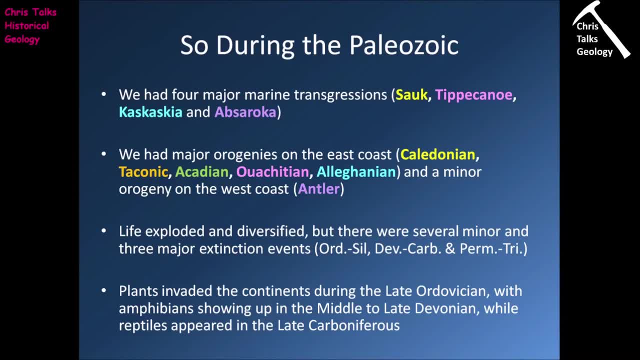 diversification of life as it begins to exploit new environments. now, as part of this evolutionary process, of course, there were several minor and three major mass extinction events. the biggest of these extinction events were, of course, the ordovician silurian extinction, the devonian carboniferous extinction and, of course, the really big one, the permian triassic mass extinction. 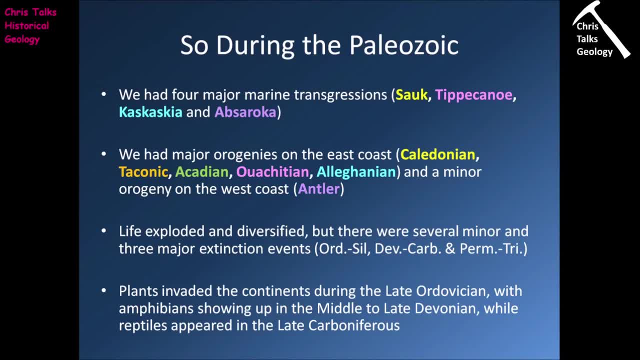 sometimes called the permotrias. now also during the paleozoic on land we had the plants invading the continents. that occurs during the late ordovician. we also see the amphibians making their way onto land during the middle to late devonian and we see the evolution, the reptiles. 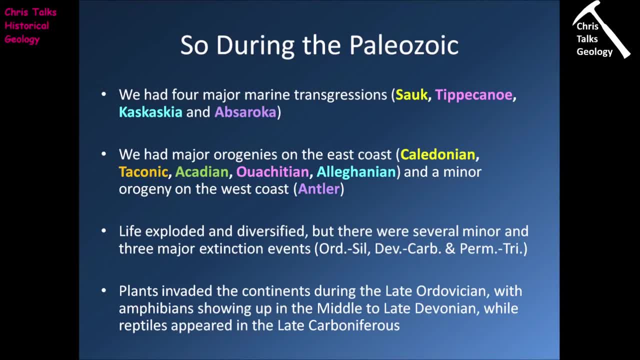 from the amphibians at approximately the late cretaceous and of course, if you remember, by the end of the permian. we're beginning to see the formation of a group of mammal-like reptiles who will obviously eventually give rise to the mammal-like reptiles. so we can see the 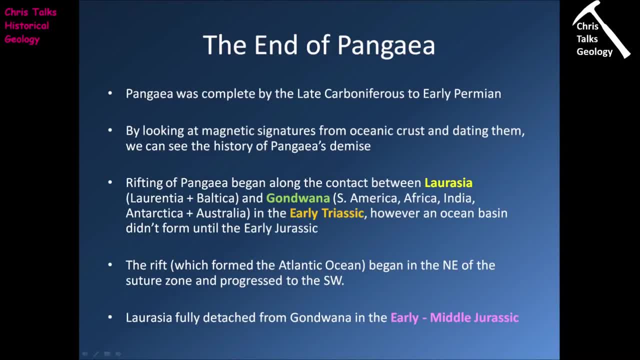 amylclade. So the transition from the Paleozoic into the Mesozoic is essentially marked by the demise of Pangaea. Now, if you remember, Pangaea was a supercontinent that completed its formation by the late Carboniferous to early Permian. Now, by looking at the magnetic signatures from 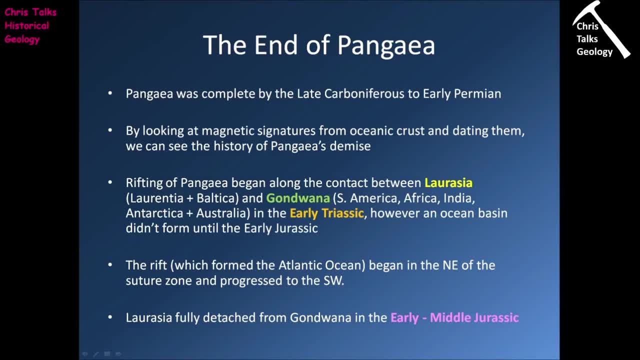 oceanic crust and dating the oceanic crust, we can actually see the history of Pangaea's demise. So what we can do is we can go out to the ocean basins now and we can take samples of seafloor rocks and we can date them, and we can also run magnetometers over the seafloor and we can look. 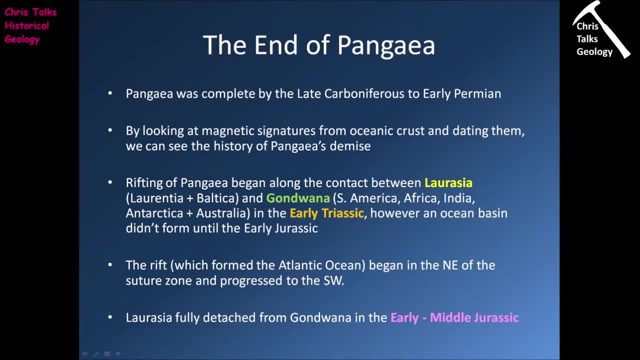 at how the magnetic signatures of the seafloor rocks have changed over time. So, if you remember, of course that's all to do with reversals of the Earth's poles. Now, what we can do with this information is by using the magnetic data we can work out the orientation of the spreading ridges. 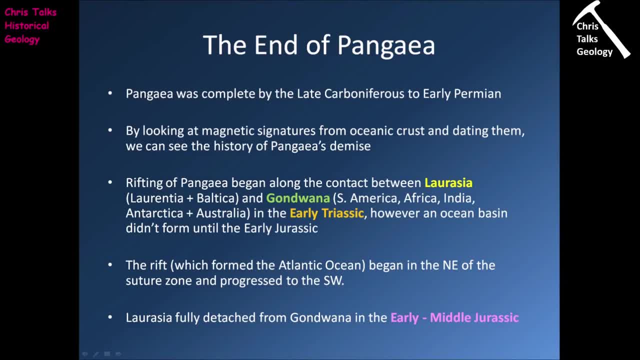 that produce the oceanic crust, Then what we can do is we can work out the magnetic signatures and we can also work out how quickly that oceanic crust has been made using the dating evidence that we have. So what we can do then essentially is we can then slowly remodel essentially what happened. 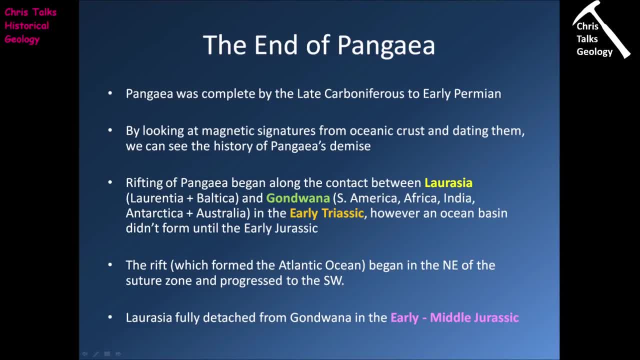 So we can use this information- the orientation, the spreading ridges and how quickly crust was being created- and essentially we can slowly, incrementally, subtract the oceanic crust and move the continents back to their starting positions. So that would have been the position of the continents during the early Triassic and then from there we can let the model run. 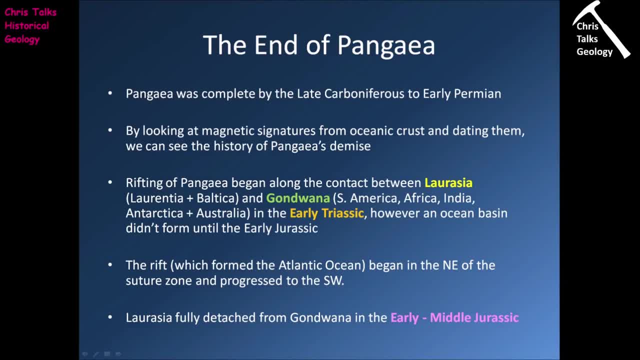 and we can see how the continents have changed over time. So we can see how the continents have moved to their current positions over time. Now, obviously, the end of Pangaea is going to be produced by rifting, the process of tearing pieces of continental crust apart. So the rifting of 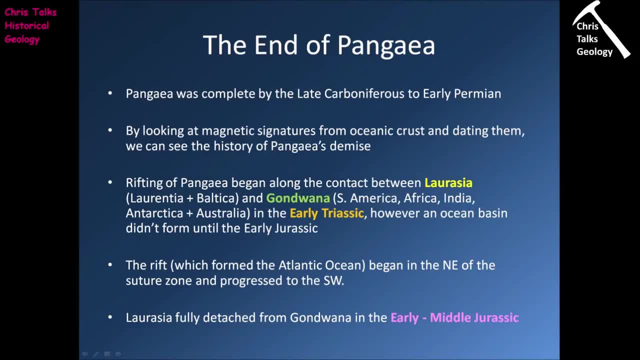 Pangaea began along what was a contact between Laurasia- so, if you remember, Laurasia is Laurentia- and Baltica- and Gondwana. Gondwana consists of South America, Africa, India, Antarctica and Australia, And this rifting started in the early Triassic. 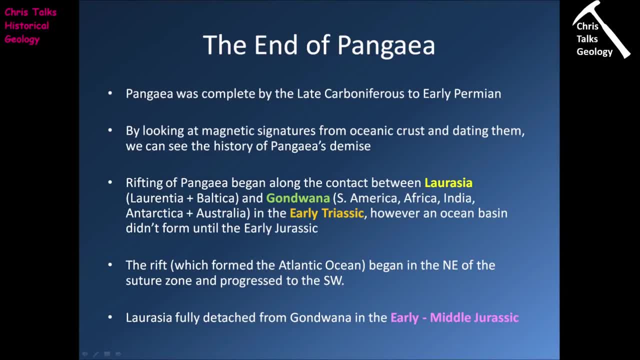 However, we don't actually begin to see the formation of a rift valley until the late Triassic and we don't see that rift valley filling with seawater until the early Jurassic. So it takes a while for an ocean basin to begin to open up. So in the early Triassic we begin to see the first. 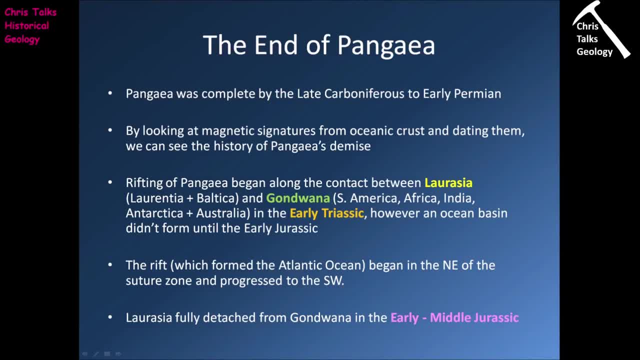 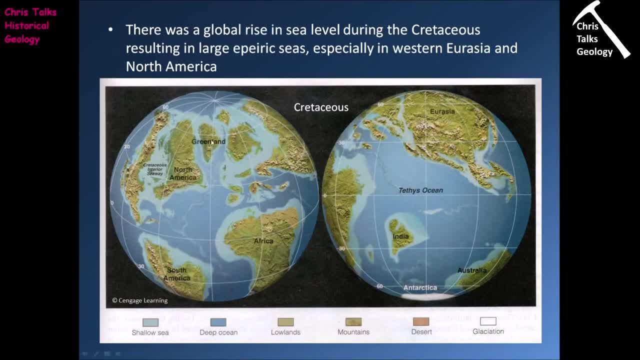 So we don't get a rift valley forming straight away. So we don't get a rift valley forming straight away, showing Greenland as a separate landmass there, and Europe is now shown as fully separated from North America here now I wish to point out that this actually 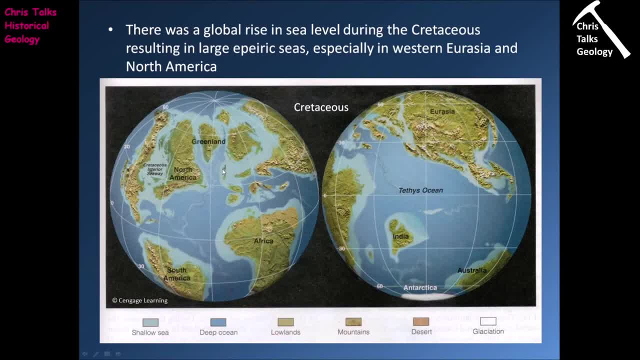 didn't happen until right at the end of the Cretaceous. so for most of the Cretaceous, North America, Greenland and Europe are still technically joined together as one landmass. it's not until literally the dying seconds of the Cretaceous that Greenland and Europe actually, you know- really begin to. 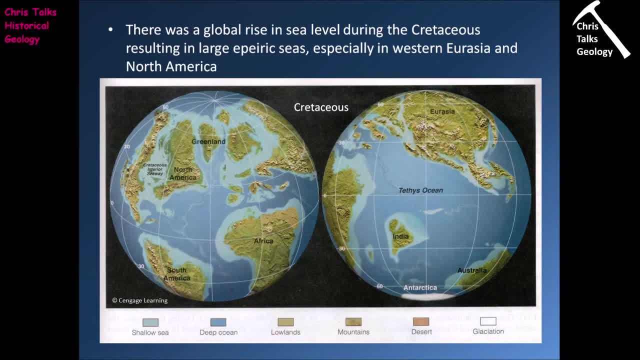 separate off from North America. now we can also see that between the Jurassic and the Cretaceous, Gondwana has completely fallen apart, so we formed a rift here between Africa and South America. obviously, this rift is going to push South America westwards and it's going to push Africa eastwards. we have a 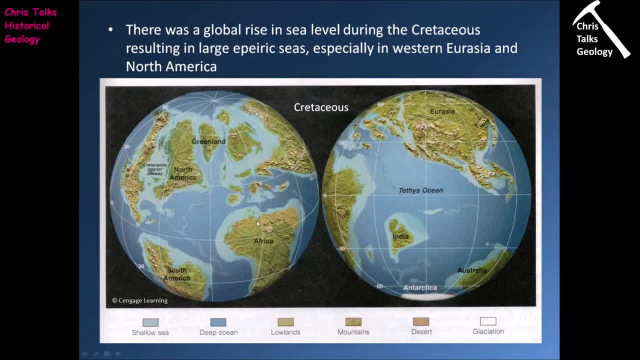 subduction zone here along the southern margin of Eurasia. that of course is going to be pulling Africa in an approximately northward direction. it's also going to be pulling India northward. so India's obviously attached to the Tethian seafloor here and the Tethian 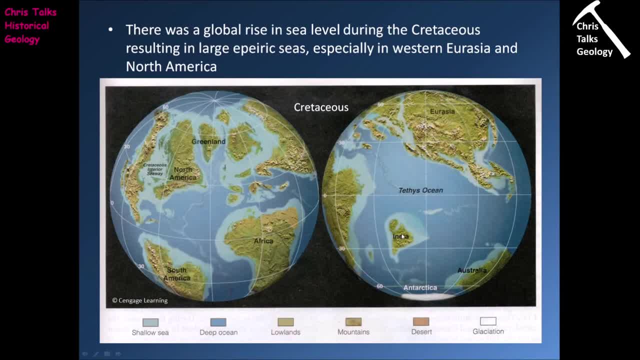 seafloor is subducting underneath Eurasia, so that's going to help to move India northwards and we're also going to have a rift open up between Australia and Antarctica. that rift is going to push Antarctica over the South Pole and it's going to push Australia off to approximately the east. now you can also 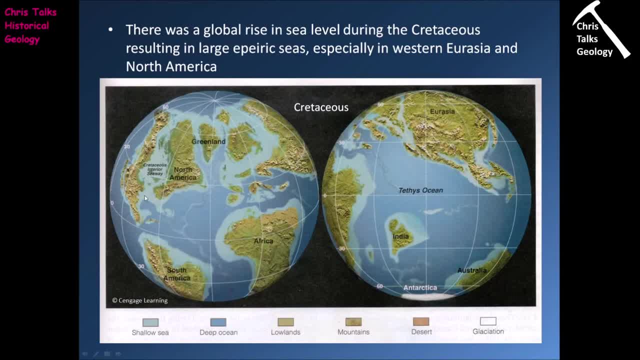 see that during the, during the Cretaceous, we also have another Epiric Sea covering North America. so we can see that there's an Epiric Sea which is stretching all the way here from the Arctic Ocean, which bisects North America and continues all. 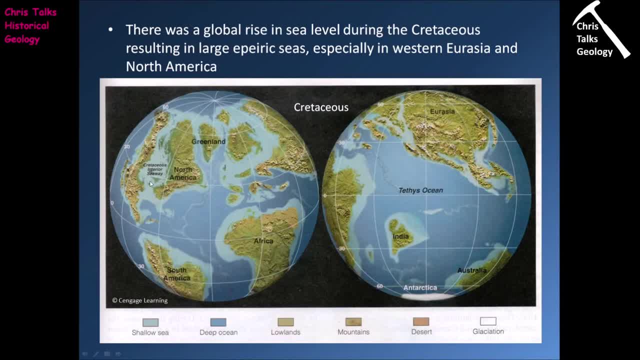 the way down into the modern-day gulf. so you know, you can see quite clearly that we have a very large marine transgressive event. however, the high ground to the east and the high ground of what is the called the Rockies to the west, essentially that area doesn't flood because of course it's elevated terrain. 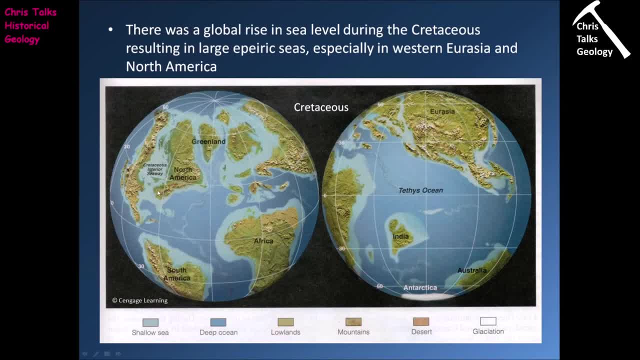 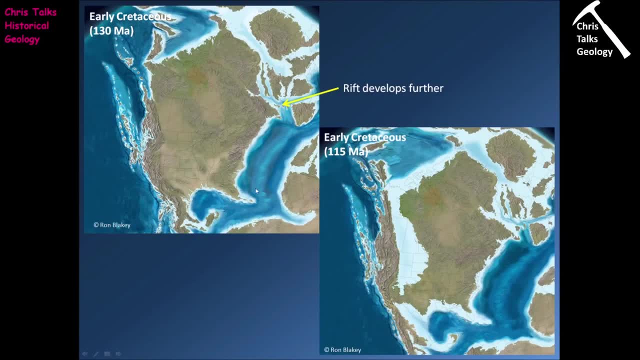 so it's only the central portion of Canada and the United States that is going to be flooded, states that really gets inundated. So by the early Cretaceous we can see that the Atlantic Basin is opening up very nicely. You can also see by this point that we have had a lot of 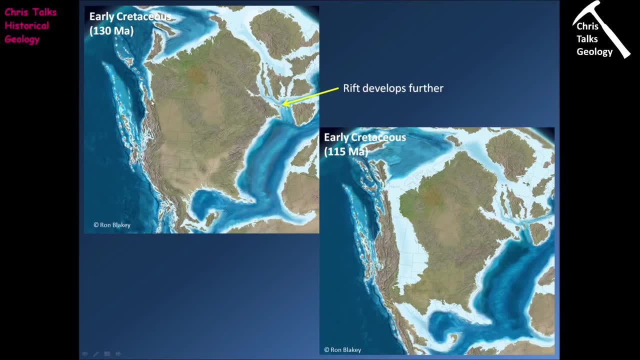 activity along the western margin of North America. We can really see the formation of the Rocky Mountains, the Sierra Nevadas, etc. Now, by the time we're into the early Cretaceous, you can see this rift here is starting to develop. We're also going to see the start of rifting. 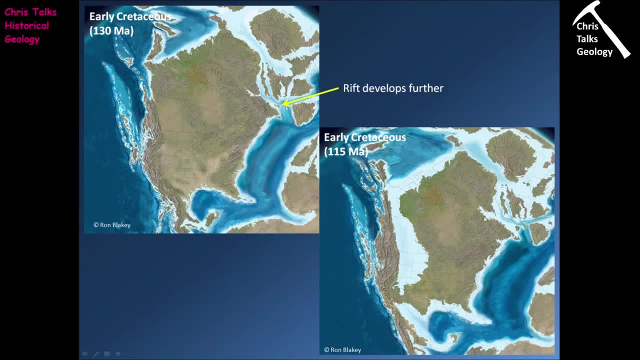 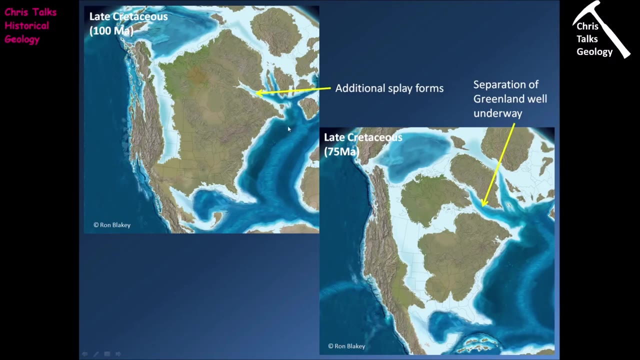 coming in from the north. So if we keep going, we're still in the early Cretaceous here we can see this rift is starting to develop even more, So it's really starting to separate off between Ireland over here, Greenland here and eastern Canada over here. And then, by the time we are 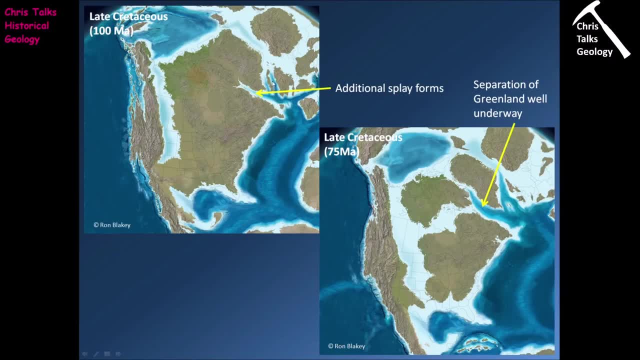 into the late Cretaceous. we can see we have this rift developing nicely, so it's moving northwards. We also have the start of a rift here between Greenland and North America By the very late Cretaceous. we can see the rift is starting to develop even more, So it's really starting to. 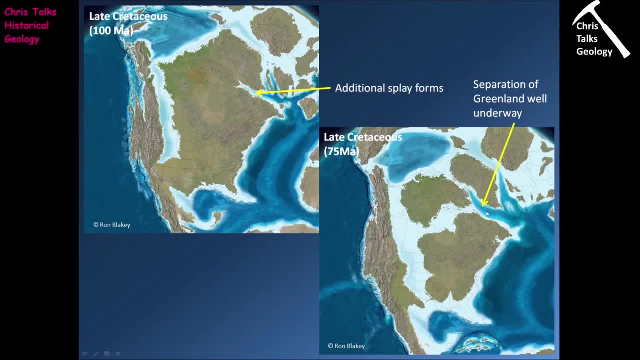 these two rifts are developing nicely. So these rifts are obviously going to eventually lead to Europe breaking off from North America and Greenland separating from North America as well. You can also see that during the Cretaceous we have this lovely subduction zone coming. 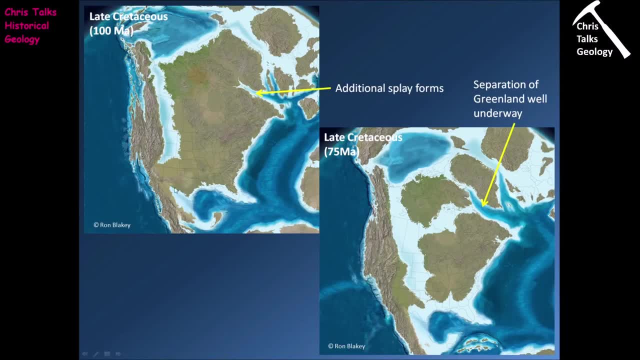 down what is now the modern day west coast of North America and Central America, And of course, we have an associated set of mountains as well, just like the modern day Andes. Now you can also see that if we just take a step back. So 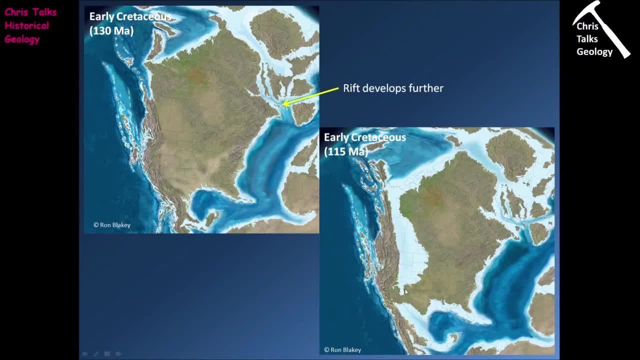 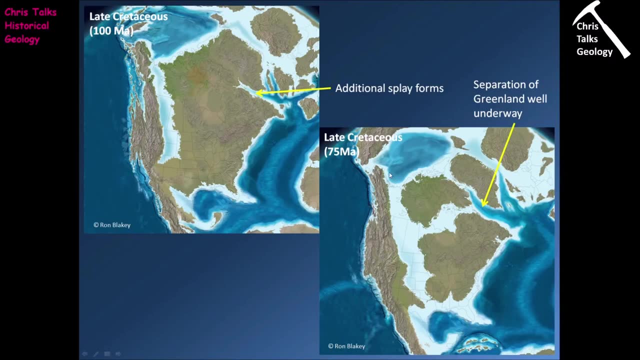 in the early Cretaceous we have the formation of a Epiric Sea here. This Epiric Sea persists into the late Cretaceous and by the very late Cretaceous we can actually see that North America is fully bisected by this body of water which is linking up the Arctic Ocean to the Gulf Coast. well, the 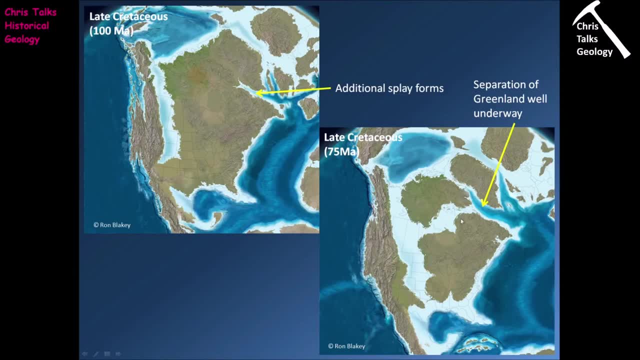 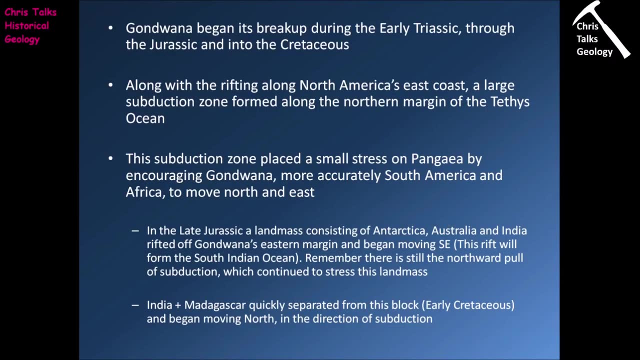 Gulf of Mexico, should I say. But we also do have another portion of the Epiric Sea here which essentially is cutting across Canada via the Hudson Bay. So Gondwana began its breakup during the early Triassic, through the Jurassic and into the Cretaceous. 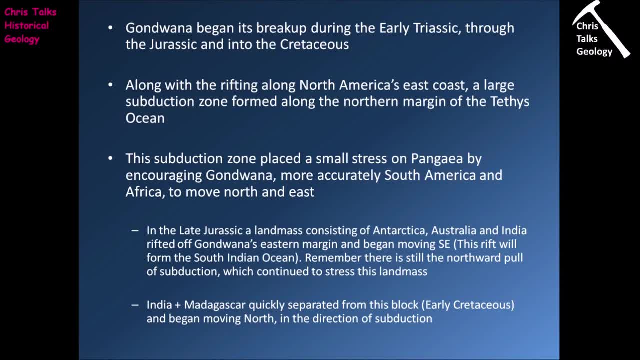 So this wasn't a fast collapse. this was a very slow and gradual process. So, along with the rifting along North America's east coast, we also have a large subduction zone forming along the northern margin of the Tephys Ocean. So we've already discussed that. the northern 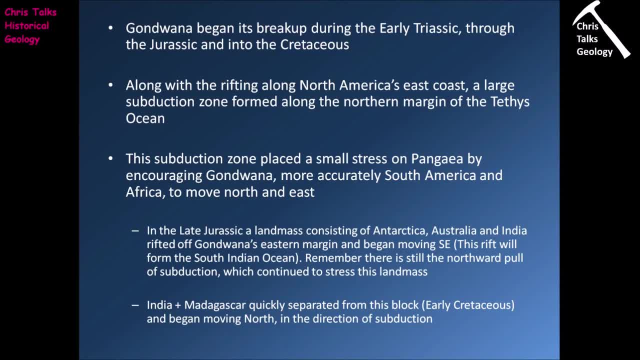 margin of the Tephys Ocean would be what we would now call the modern day south coast of Asia. Now this subduction zone placed stresses on Pangaea, So Pangaea, of course, was breaking apart and of course the rift between Laurasia and Gondwana was trying to push Gondwana approximately eastwards, but at the 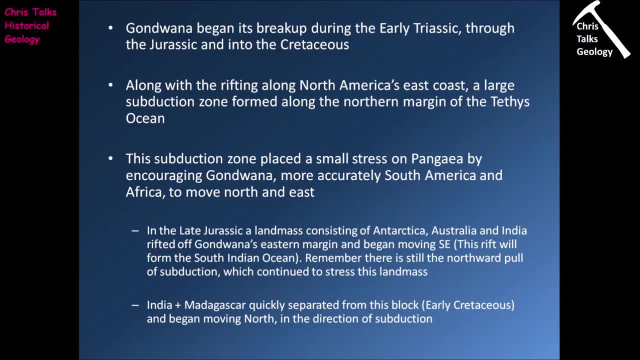 same time, you have this northerly pull from this subduction zone and of course that means you're trying to essentially push one side of Gondwana one way and pull the other side another way, and that's going to start stressing the supercontinent of Gondwana and that's going to help to contribute. 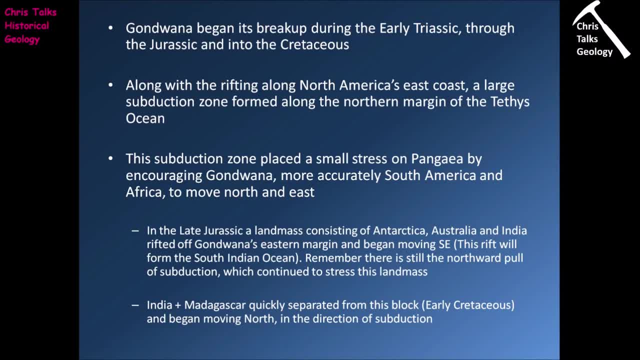 to its breakup. Now, in the late Jurassic, we see a landmass consisting of Antarctica, Australia and India rifting off Gondwana's eastern margin and, of course, this landmass. so this Australia-India Antarctica landmass begins to move to the southeast. 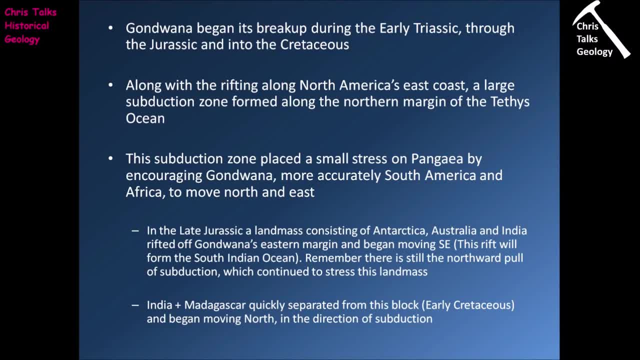 and this rift will form the southern Indian Ocean. Now we also need to remember there's still this northward pull, though, so this rift is pushing this landmass consisting of Antarctica, Australia and India in an approximately south-easterly direction. however, at the same, 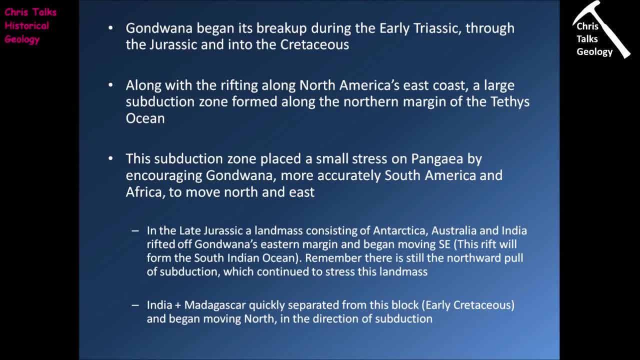 time that landmass is also being tried is also trying to be pulled to the north by the subduction zone. This, once again, is going to result in this landmass becoming stressed and eventually breaking up. So this stress is eventually going to lead to India and Madagascar separating pretty quickly. 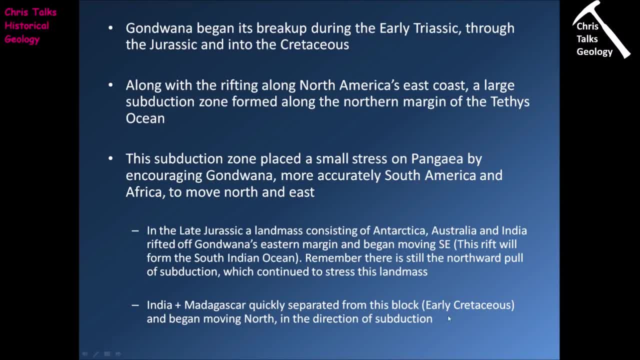 off this landmass, and this is going to occur in the early Cretaceous and, of course, there's going to be a rift forming between India and Madagascar. This rift is going to obviously push Madagascar westwards towards Africa, whilst India is going to move northwards because of this subduction zone. 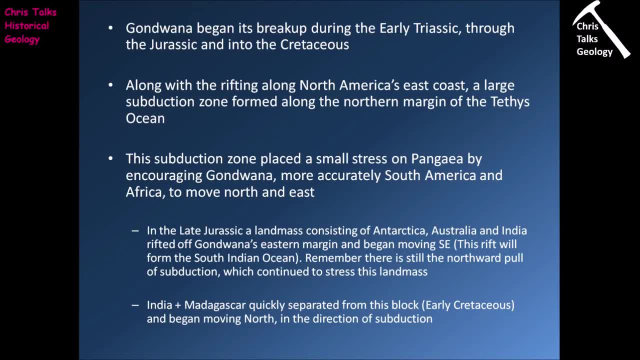 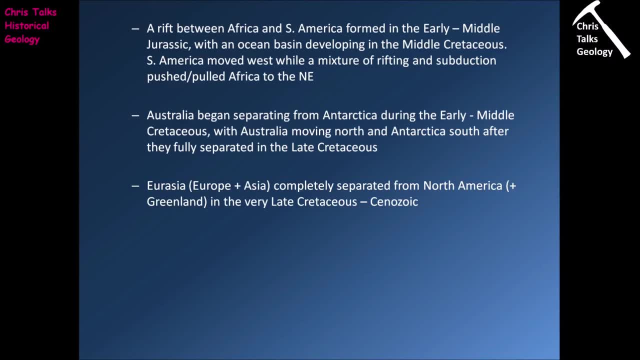 along the northern margin of the Tethys Ocean. We're also obviously going to see a rift between Africa and South America forming, and this is going to begin in the early to middle Jurassic. so this is going to come after the formation of the rift that comes along the east coast of North Africa. This rift is going to be a rift between India and 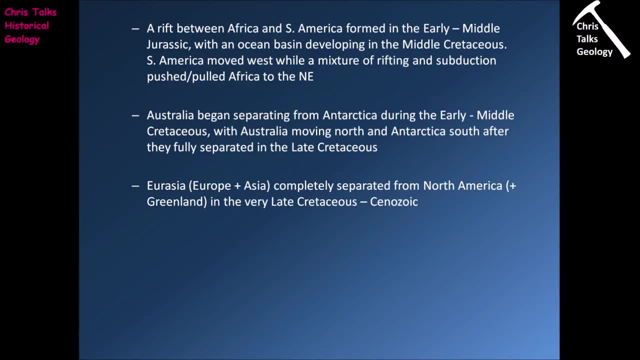 North America and, of course, this is going to develop into an ocean basin by the middle Cretaceous and of course, this is what we call the South Atlantic Ocean. Now, the formation of this rift is, of course, going to push South America westwards and Africa eastwards In terms of 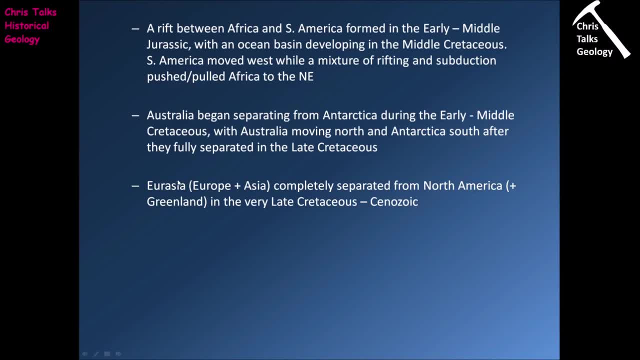 Australia. it actually stays attached to Antarctica for a very long period of time and we begin to see the first stages of its separation from Antarctica occurring in the early to middle Cretaceous, and the second stage of its separation from Antarctica, The rift zone that forms in between. 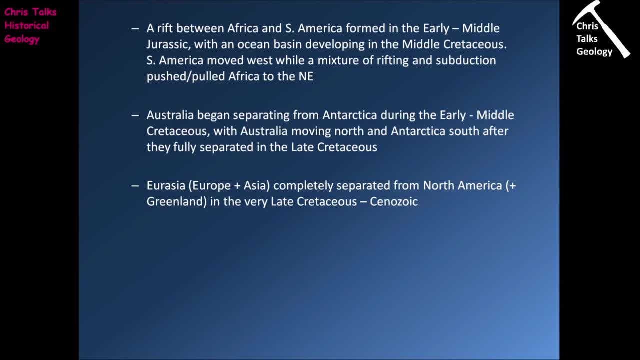 them is going to push Antarctica southwards to its current position over the South Pole, and it's going to push Australia in an approximately east-north-east direction. so it's going to move it towards its current location In terms of Eurasia. so that's Europe plus Asia. it's going to stay. 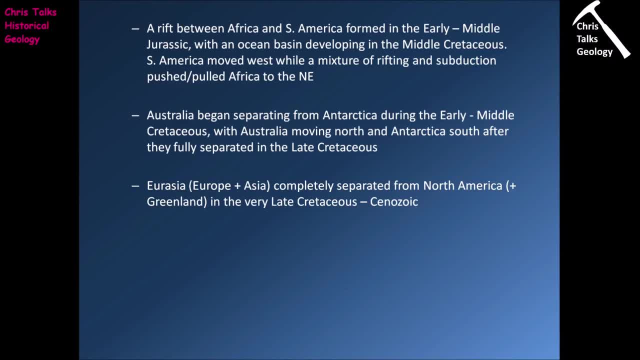 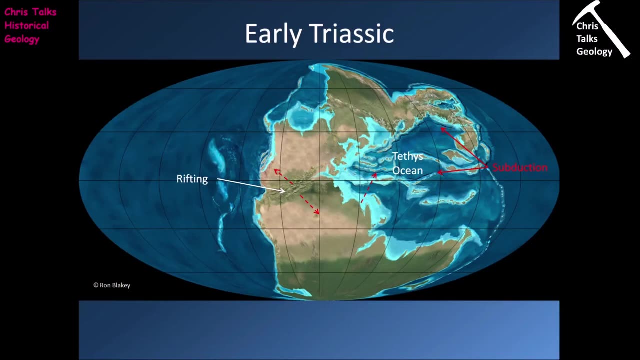 connected to North America for much of the Mesozoic and we are only going to see Eurasia separating North America in the very, very late Cretaceous. Okay, so what we're going to do now is we're going to look at some global maps for the Mesozoic. 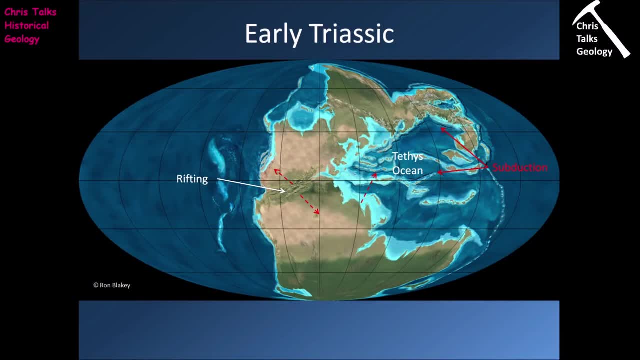 and we're going to try and see how the continents are moving relative to each other as we go from the Jurassic into the Jurassic and then, of course, into the Cretaceous. So what can we see when we look at this map? Well, obviously, we can see three main things. 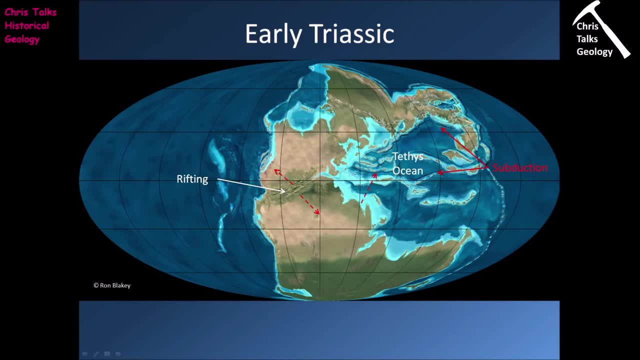 First of all, we can see the supercontinent of Pangaea. we can see the Tethian Ocean Basin over here and we can see the Panthalessic Ocean Basin over here Now, in terms of Pangaea itself. so obviously North America is going to be about there. Europe is right here. 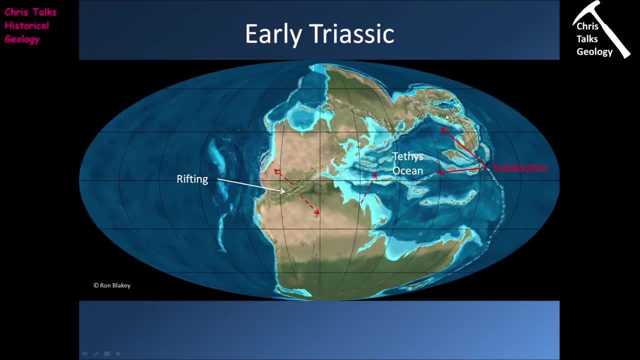 Central Asia is about here, Southeast Asia is going to be over here, we have South America there, Africa is going to be here, India is about there, Australia is over here and Antarctica is going to be over here. So what we're going to do now is we're going to try and see how and why these 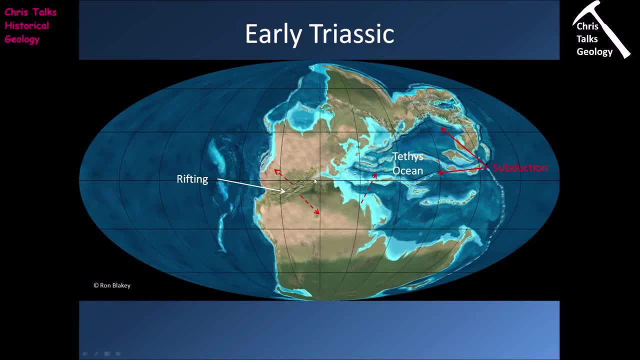 continents are moving relative to each other. So the first thing we're going to notice is we can see the rift beginning to form between North America here, South America here and Africa here, and of course this is going to give us the Atlantic Ocean Basin. So the rift itself is obviously trying. 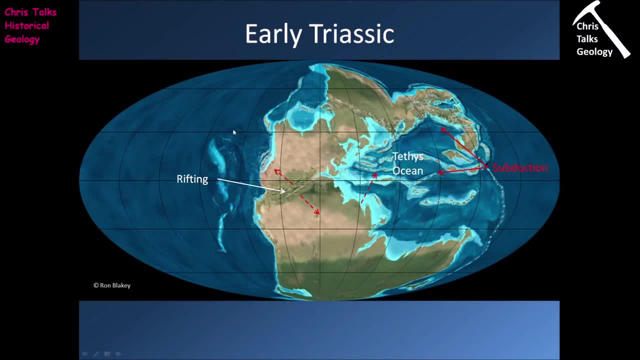 to push North America off approximately to the northwest, and it's trying to push this southern, what we would call Gondwana, down to the southeast. Now, at the same time, if we look over here at the Tethian Ocean Basin, we can see we've managed to establish a couple of subduction zones, one here: 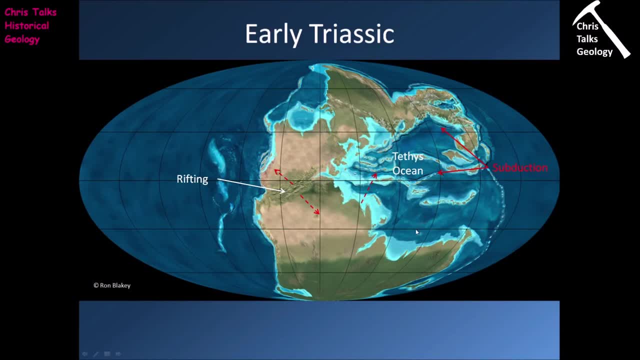 and one here, and so they're going to be taking the oceanic crust here and they're going to be subducting it northwards underneath what will become Asia. So the oceanic crust here is, on a whole, moving in an approximately north easterly direction. so 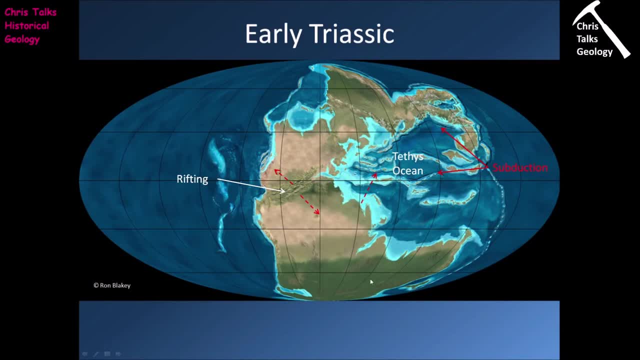 Gondwana. this continent down here, consisting of South America, Africa, India, Australia and Antarctica, is trying to both move to the southeast and to the northeast, so it's being pulled in two different directions. The other thing you'll notice is that we also have a subduction zone. 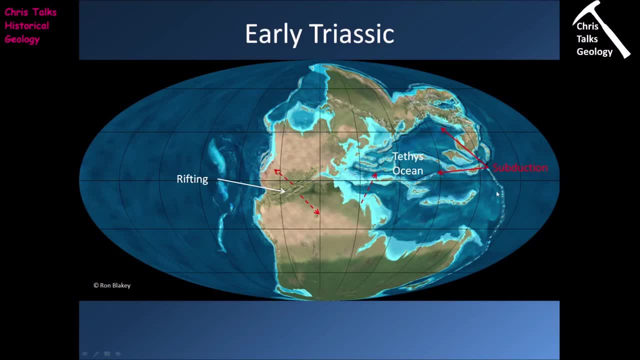 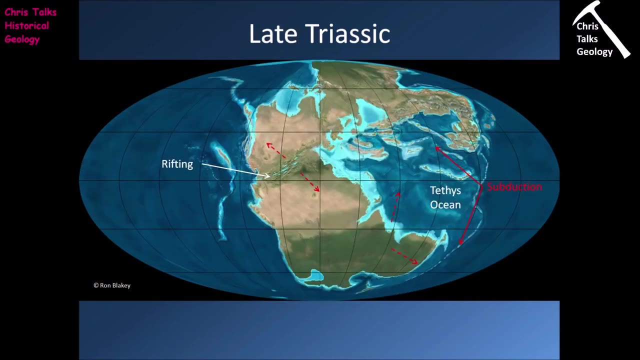 right here along the eastern boundary of the Tethian Ocean Basin, and of course that's also going to encourage the entirety of Pangaea to want to move approximately eastwards. so you can see, we have going on here. Okay, so by the late Triassic, what have we got now? Well, we can see. 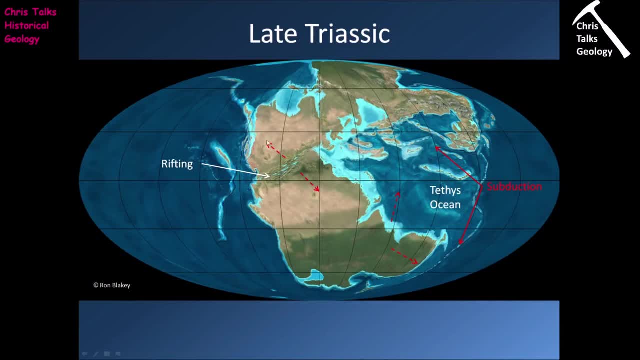 the rift is opening up nicely and we can see we're getting a bit of separation between North America and South America and Africa. now We can still see of course North America, Europe and Asia are all joined together. We can see that the subduction zone is still established along the northern 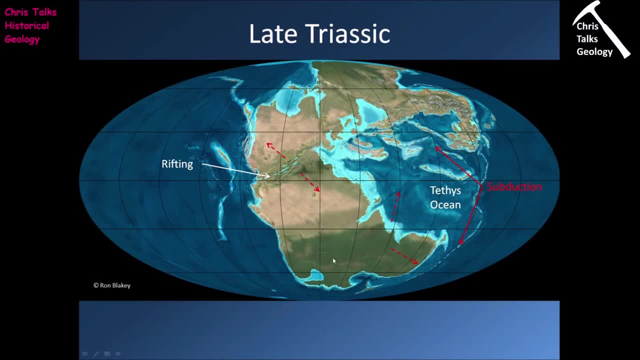 boundary of the Tethy and Ocean Basin and of course that's going to be trying to pull the mass of Gondwana northwards. This rift here is going to be trying to push Gondwana to the southeast and so once again, we have this continued double pull, essentially on the 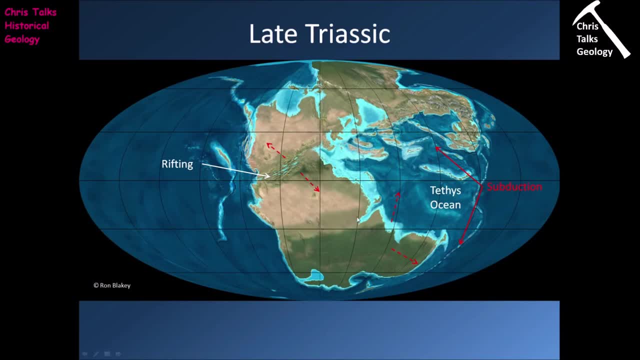 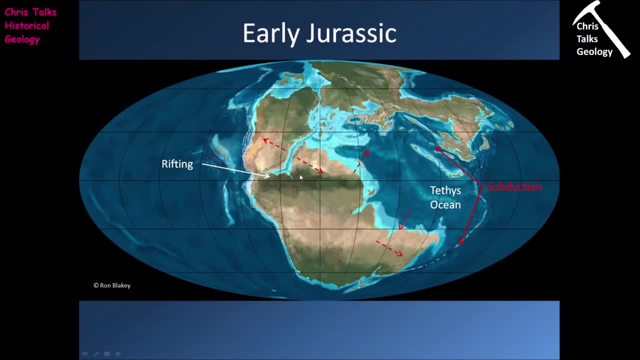 continents down here. So we're stressing the supercontinent of Gondwana in two different directions. So as we move into the early Jurassic we can see we now have complete separation between North America and Gondwana, So we have an almost complete. 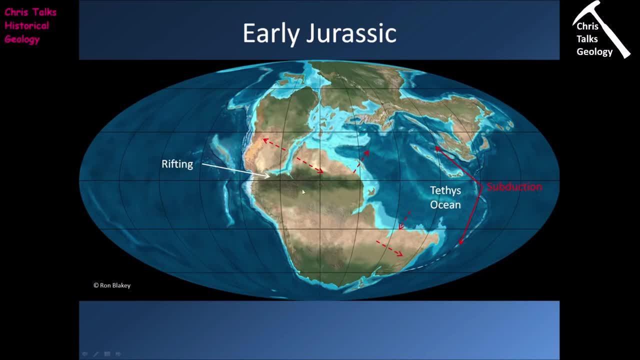 rift between North America and Gondwana, So we have an almost complete rift between North America and Gondwana. So we have an almost complete rift between North America and Gondwana, So which of course, looks like it's going to be a bit more transition here along the northern Bison. 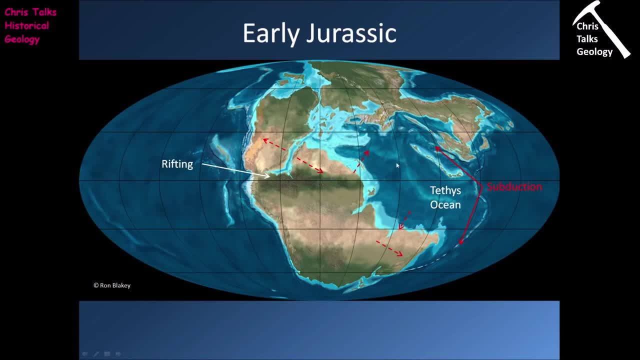 forming here. Subduction zone is still operating along the northern margin of the Tethy and Ocean, so it's still trying to move Gondwana to the northeast. Now we have a. we have a spreading ridge right here and this is going to be obviously creating oceanic crust. It's going to be trying to 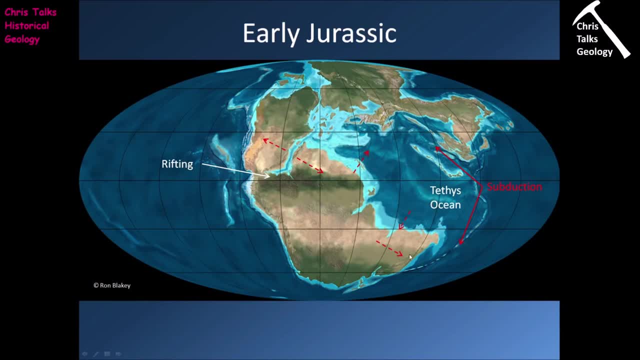 push this area of oceanic crust down towards the southwest and obviously this area is going to continue off towards the north northeast. We have multiple stretches of the bariocephaly on either side of where I is placed. I see Tethy setting a full preparation date. 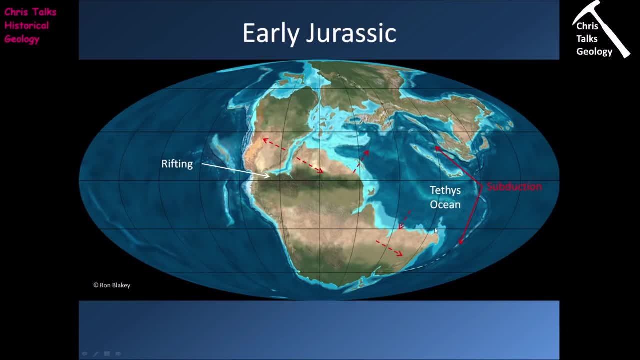 is now. We have one stress that's trying to push Gondwana southeast, we have one stress that's trying to pull Gondwana towards the northeast and we have another stress that's trying to push Gondwana towards the southwest. So I think we can agree: this isn't going to end well for Gondwana. 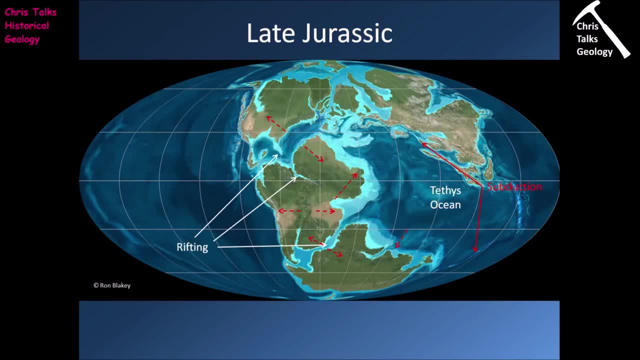 So by the late Jurassic we've started to see the complete and total disintegration of the Gondwanan super continent. So we can see, initially we have a rift valley opening up here between Africa and South America on one side and India, Australia and Antarctica on the other. 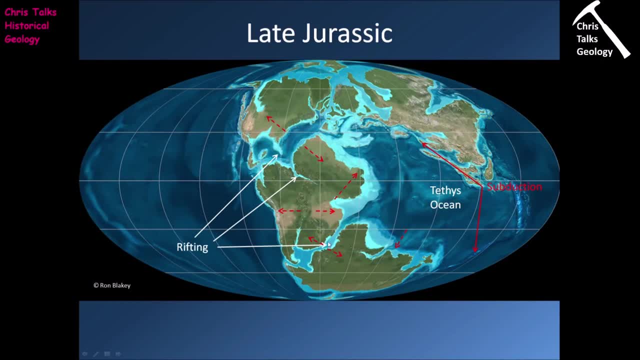 and of course, this rift valley here is going to develop into the Indian Ocean. We can also see at the same time we have the start of rifting between South America and Africa, coming from both the north and the south simultaneously, and we can begin to see we have the start of rift forming here. 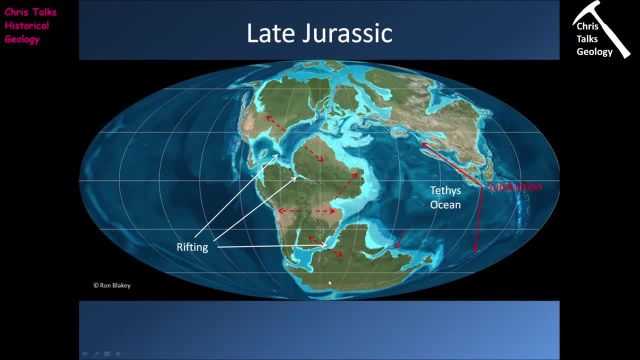 which is the result of a rapid drift between the two sides of the continent, is going to allow India to separate off from Antarctica and Australia. So the subduction zone here along the northern margin of the Teffian Ocean Basin is still active. The spreading ridge. 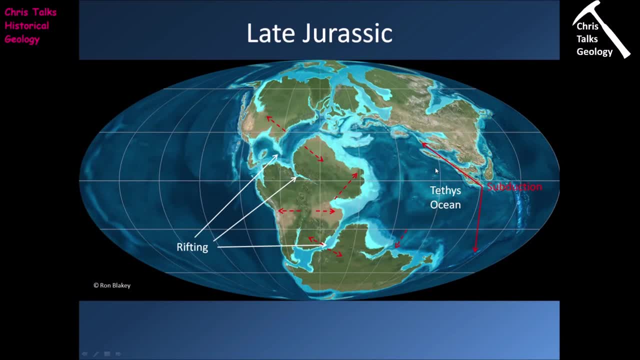 that was here is slowly moving northwards towards that subduction zone. We can see the Atlantic is starting to get larger. We can see we've now established what it looks like the east coast of North America. here We can see we have the Gulf of Mexico forming there and we can even begin to 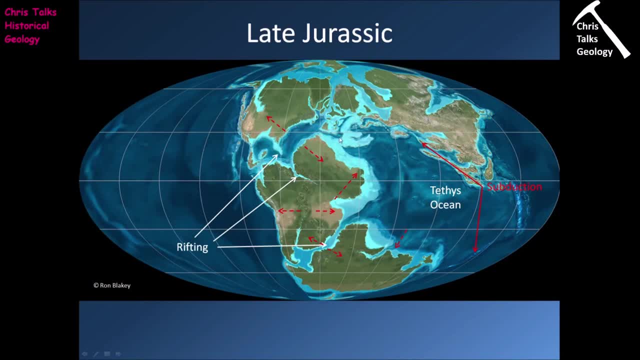 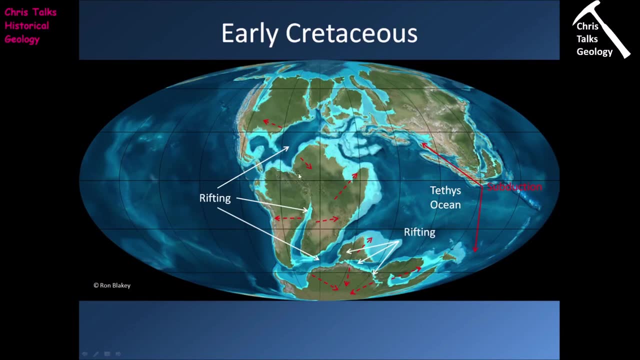 see a bit of rifting here in what will become the modern day Mediterranean Ocean Basin. So as we move into the early Cretaceous, we can see the rift between South America and Africa is extending. It's nearly complete. it's not quite there. We can see at this point the rift which was 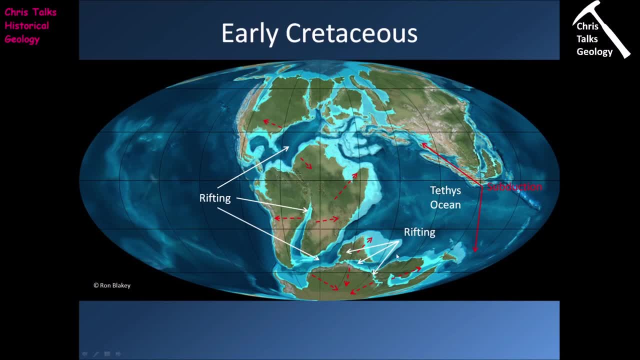 starting here, has progressed and essentially it's progressing. It started originally by going southwards. now it's turning westwards and this is allowing India and Madagascar to rift off the other landmass consisting of Australia. So, as you can see from this diagram, we can see we have lots of different forces all operating. 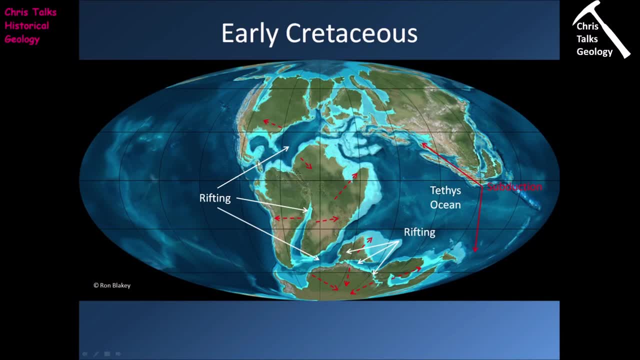 simultaneously now. So we have the spreading in the North Atlantic which is obviously trying to take North America off to the west and it's trying to push Africa and South America off to approximately the southeast. The subduction zone is still active here in the Teffian Ocean Basin. 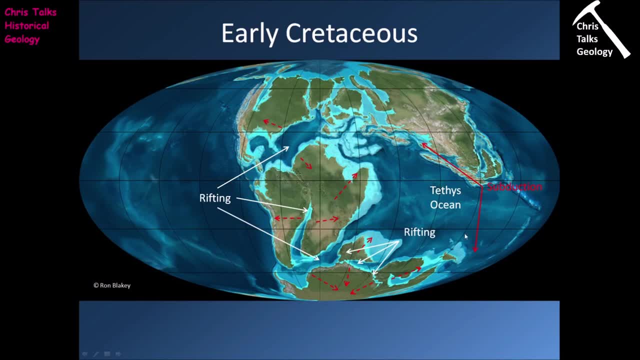 That's trying to pull Africa northwards at the same time as it's being pushed eastwards. We have the rift here Between South America and Africa. that's trying to push South America westwards and Africa eastwards again. You can see we have this rift here between India and Antarctica. Now India of. 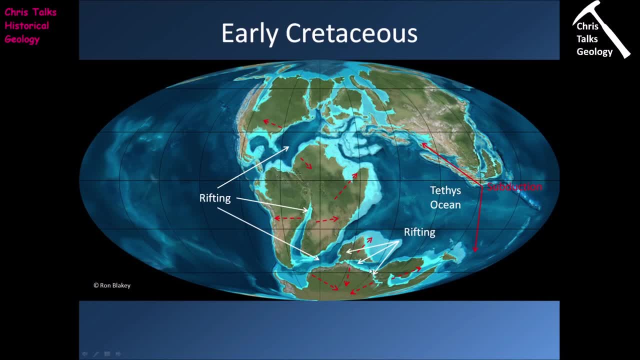 course, wants to start moving northwards. It's being pushed by both the spreading ridge here, which is pushing it northwards, and the subduction zone here is pulling it northwards. So India is going to start moving northwards at a very, very rapid rate, And we can also see- we have the start. 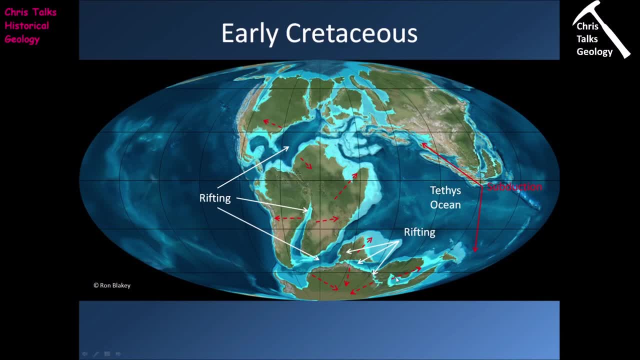 of a rift forming here between Antarctica and Australia. That's going to obviously push Antarctica- as Australia sorry- approximately northwards, and it's going to move Antarctica towards the south pole, And so by the time we make it into the late Cretaceous, we can see that. 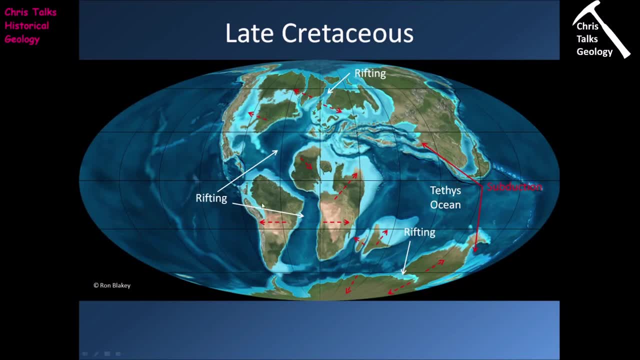 all the continents are pretty much separated from one another. now We can see South America is now fully separated from Africa and we have the South Atlantic Ocean established there. We can see that we now have the Indian Ocean growing here. We can see the Teffian seafloor is still being subducted. 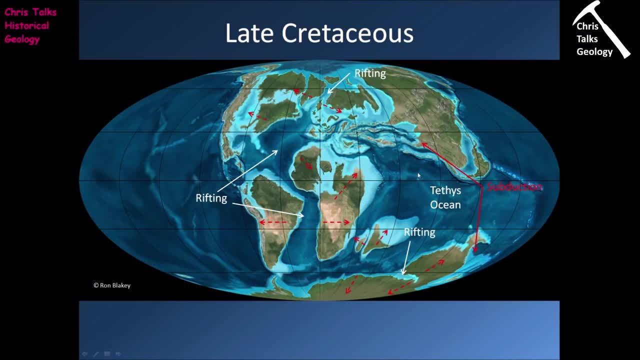 underneath Asia. The spreading ridge is now about here and it's probably not too long for the world. It's almost about to be subducted. We can see the rift here is extending between Australia and Antarctica and they'll separate right at the end of the Cretaceous And we can see the rifting that's being established.